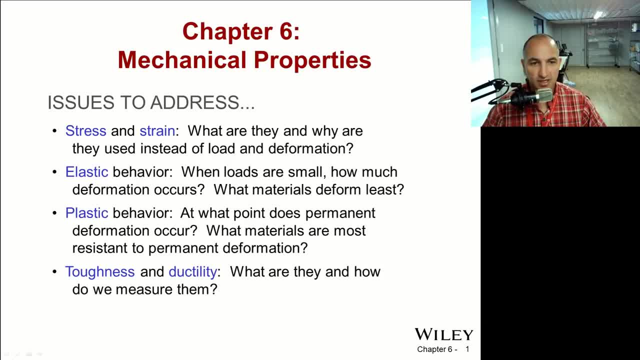 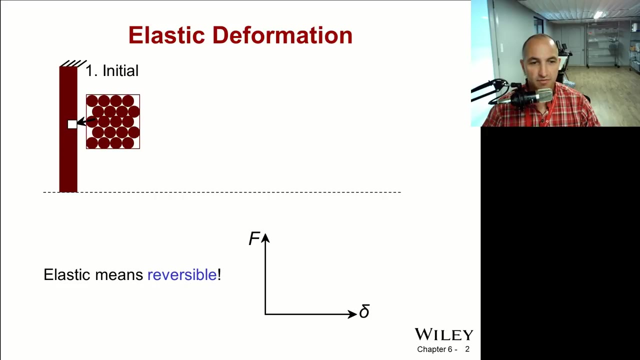 Plastic behavior. At what point does permanent deformation occur? What materials are most resistant to permanent deformation? Finally, toughness and ductility: What are they and how do you measure them? So let's get started. Plastic deformation is deformation that is reversible, or plastic-meat reversible. 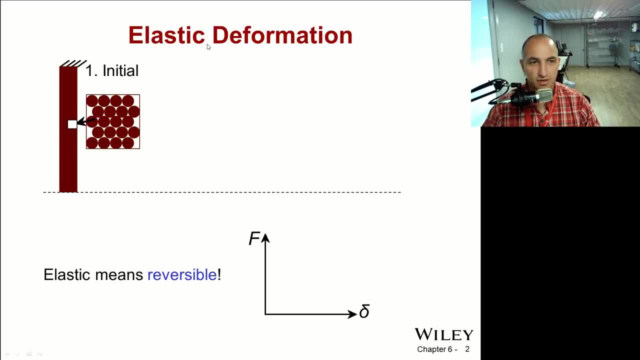 So, starting out with an initial sample here, it's a bar, a certain length. This is cross-sections blown up showing atoms stacked on top of each other. Now if we extend the length of of that bar by a count, delta pulling on it with a force F, the atoms looking at them very close up. 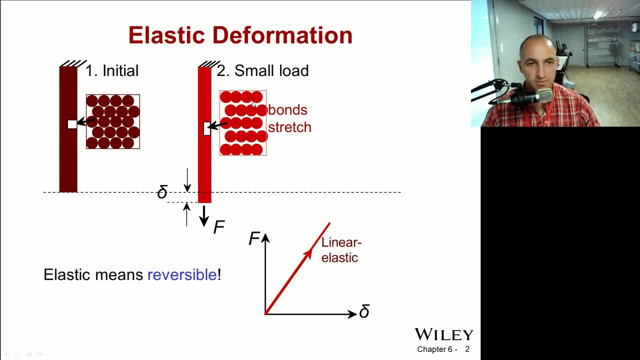 we start to see gaps between the faces of the atoms in a longitudinal direction, and so the bonds are stretching. So if you look at the force versus delta or this amount here we are in a linear elastic where force increases to delta. 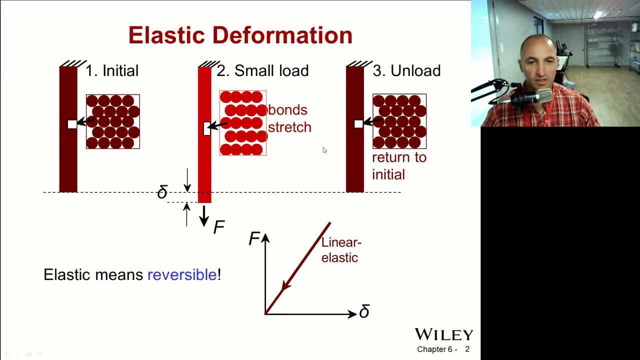 Now, if we release the load on the bar again, it returns to its initial shape and brings the atoms or those bonds bounce back. It's back to where it was. So that's elastic deformation which is reversible. 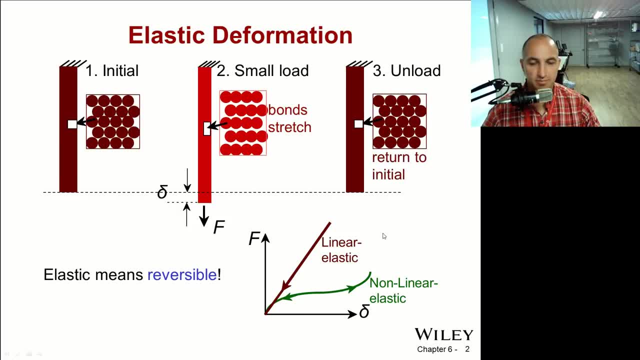 Now, on the other hand, there might be different types of materials, not all materials. We might have materials that are non-linear elastic. so rubber bands or certain stretchy materials have that behavior. So that is a non-linear elastic. Try stretching a rubber band the next time you have one and see if you can get a sense of how that force changes. 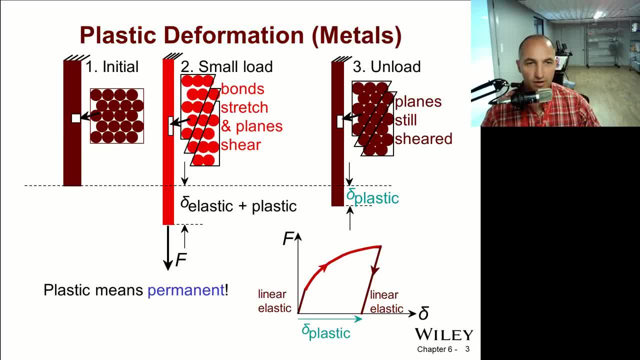 with distance. Now, if you were to stretch the sample even further, you would not need elastic. Now, if you were to stretch the sample even further, you would not need elastic deformation. start to get what we call plastic deformation. plastic deformation per minute. 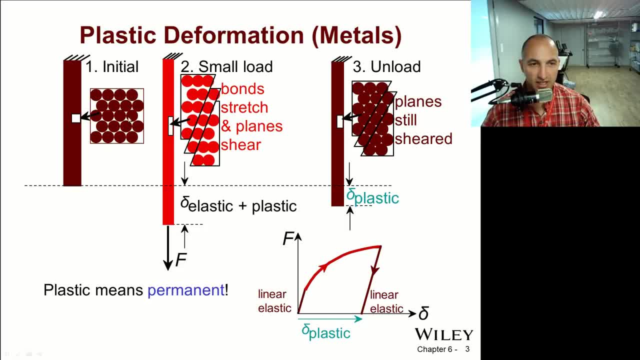 so the sample starts out initially here, at number one. we stretch the sample and first the bonds start to stretch and at some point start getting planes shearing and going back to what we learned about dislocations. that's what's occurring here: dislocation, motion, and the total distance for delta is much greater. 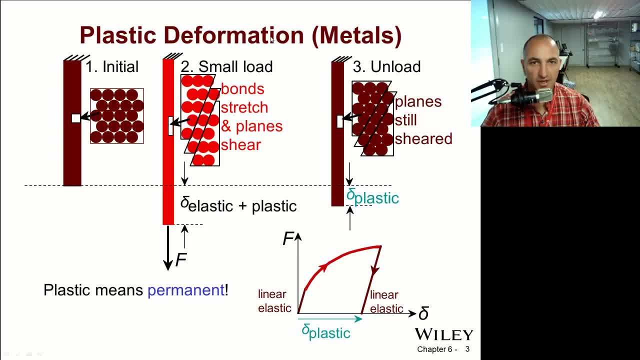 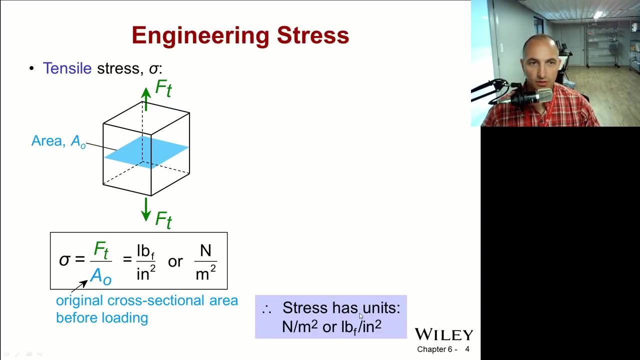 so this behavior is very common in metals. by the way, when we unload the sample, the plastic deformation remains. plastic deformation remains, but the elastic deformation does not. it returns back to its original state. so that is what happens here: when the force on it- so there's a new term here is called engineering stress. 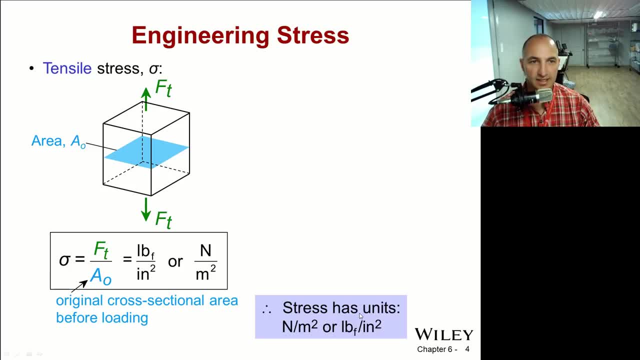 so engineering stress is tensile stress sigma and it's equal to the force that's applied to a area perpendicular to it. so force is green area, a knot. and so a knot is not because it's called the original cross-sectional before loading. as you pull on it, a knot is actually going to be decreasing. 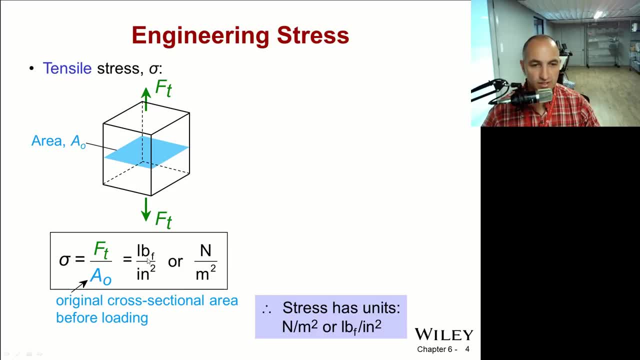 so this is the original and the units for this are pounds per square inch or newton per square. so those are the units for stress and you may also have agreed that this metal sample is going to experience if the force not apply to the cross-sectional area and we're looking at so 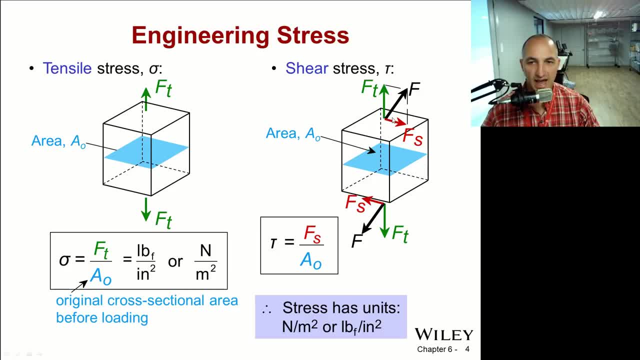 So if the force is now black line F, you have a component that's tensile and you have a component that is shear, that's perpendicular to it. So shear stress is just F sub S over A naught, And the units for shear stress are Newton per meter squared or pounds per inch squared. 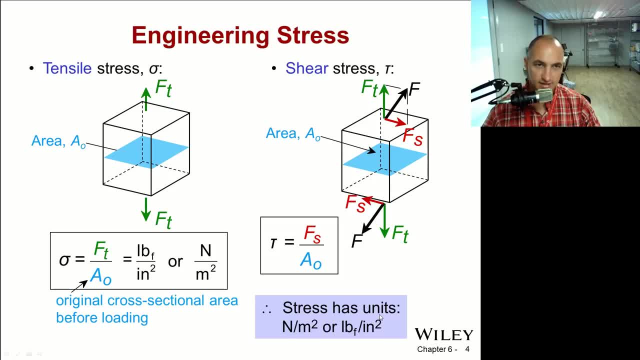 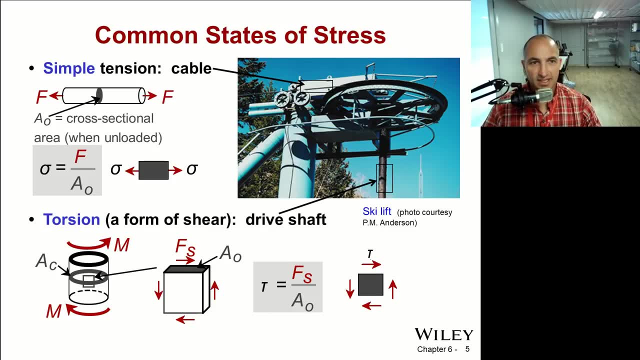 So, the same as There are some common states of stress, There is a simple tension. This is synonymous to a table on a T-lift, for example, where all of the stress is launched to the direction And the stress is just F over A naught. 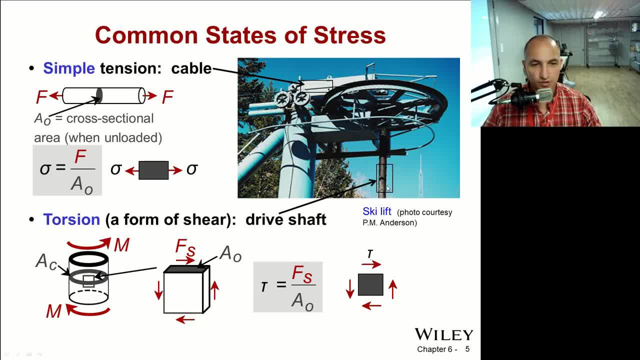 Also in the ski lift you might have proportional stresses And on that axial shaft, if you look at the component here, everything is here. So F sub S over A naught. So you have shear stresses in plane and out of plane. 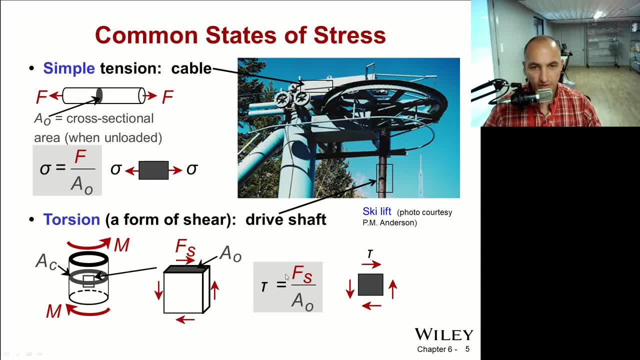 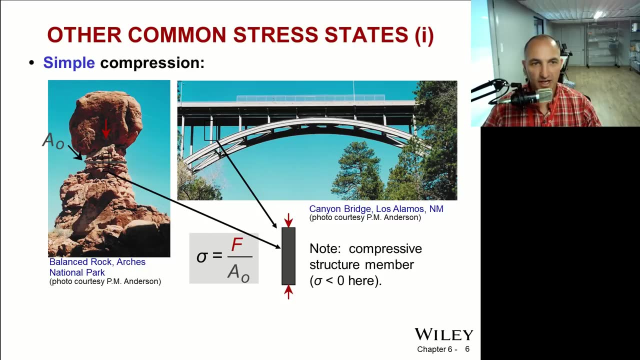 So the shear stress for torsion is just F sub S over A naught. So that's torsional. Other types of stress states have simple compression. This is similar to tension, But now we are talking about torsion, So we are talking about torsion. 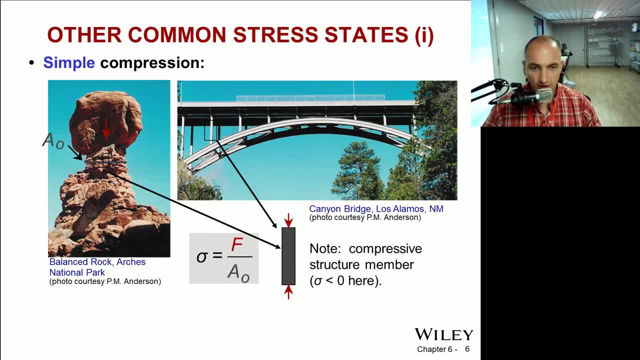 So we are talking about torsion. So while compressing the sample, there are no shear stresses in this case either. So sigma is equal to F over A naught. Here are some examples of simple compression: On a bridge being here, and on this balancing rock in the part you see on the chart. 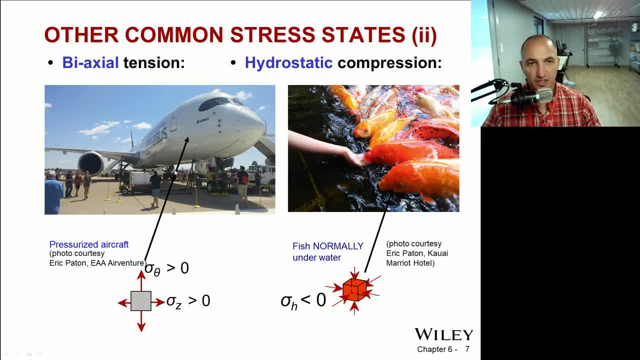 Another type of common stress state we have biaxial tension. this is actually a picture that I took while I was at the Oshkosh air show a couple years back, and this is an A350 Airbus, a new aircraft that is almost all carbon fiber composite. 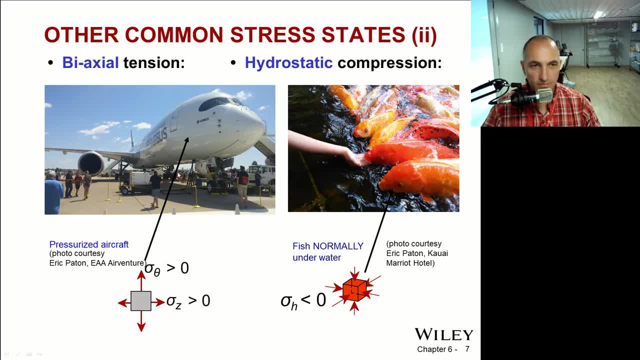 so the stress in the skin of this airplane is called the biaxial tension. so another type of stress is hydrostatic stress, and this is a picture that I took while feeding the ferocious koi at the Koi Marriott Resort, and they were literally out of the water. 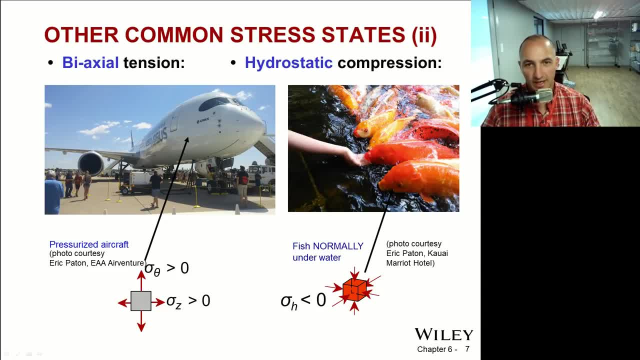 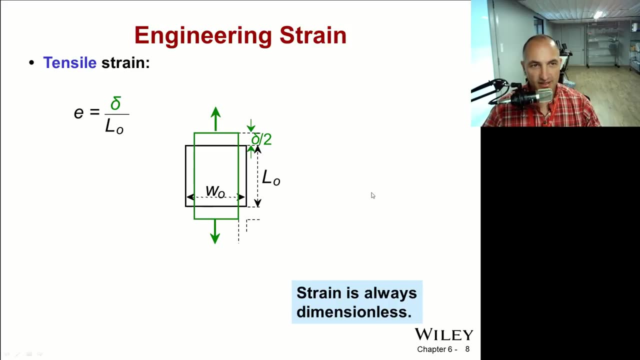 to get food. so these are not following the rules of hydrostatic depression. they're probably experiencing a lot more in their belly, all right. so engineering strain- another term that we're going to pick up, and this is tensile strain, which is epsilon- is equal to delta over L0. 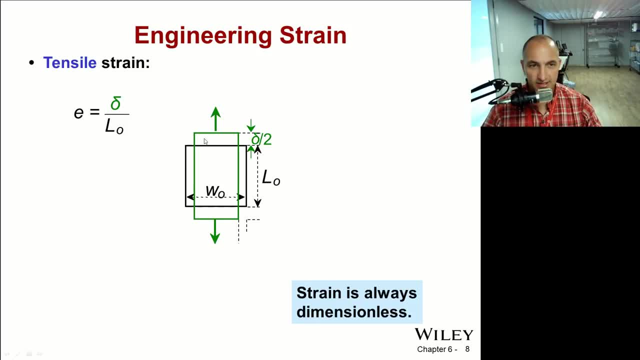 so that's the change in length over the original strain. we call that tensile strain, and strain is a dimensionless parameter. here you can see it could be in, you know, meters over meters. that's going to be dimensionless. the lateral strain is the change in dimension. 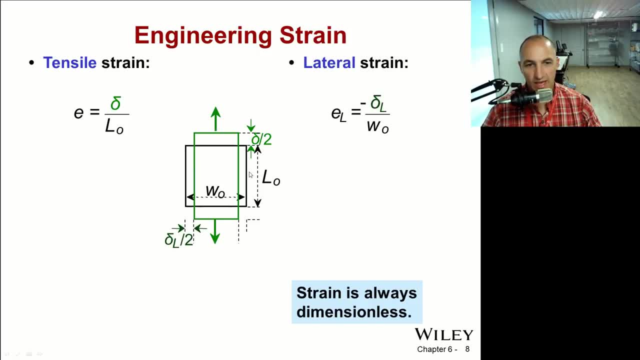 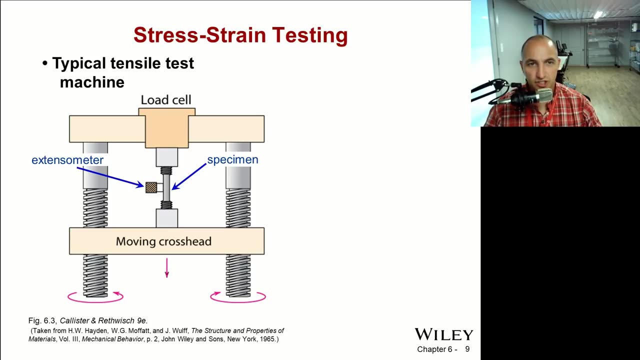 change in the dimension in the lateral direction. so that's a negative delta sub L over the original width or W0. so we measure tensile stress, tensile strain apparatus like this: it has a load cell on the top and it has these giant screws which start to pull the sample apart. 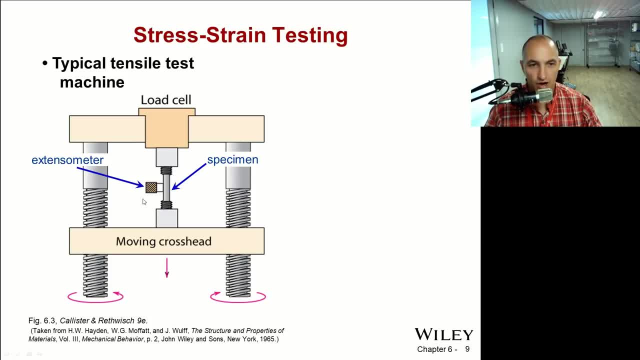 like a pre-machine bar with threaded ends on it. then there's an extensometer which is attached to it, which measures increase in length, for example- and here's a typical tensile specimen here- and it's important to have a consistent diameter across the length of the speech. 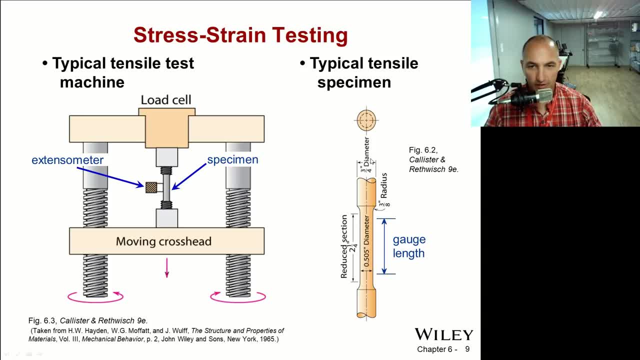 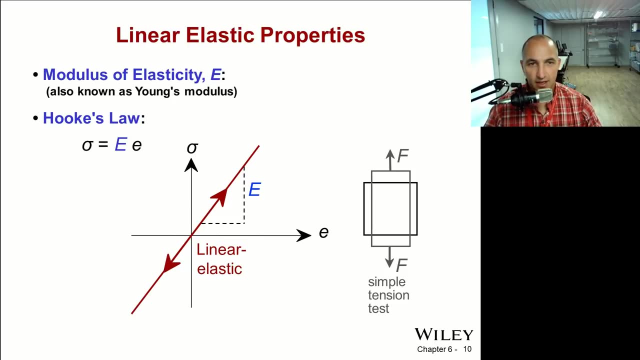 and that way we can also calculate the A sub knot for the cross-sectional area that the force is applied to. there are linear elastic properties- another term to bring up- and there's a material property called the modulus of elasticity, also called the Young's modulus, and this 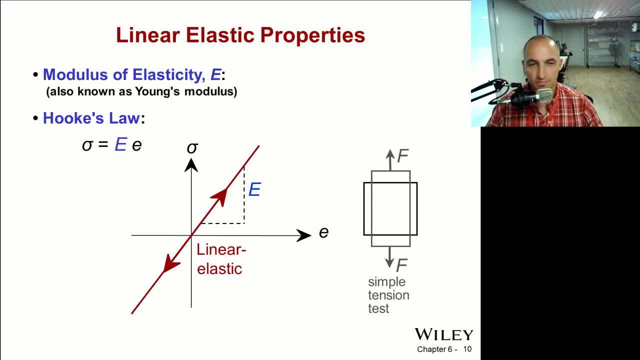 is. we also refer to this as stiffness, or the strength of the bonds between the atoms while it's, while it's being stretched to the elastic region. so this is the early stress before it starts to deform, and in metals this is typically linear and so we can measure. 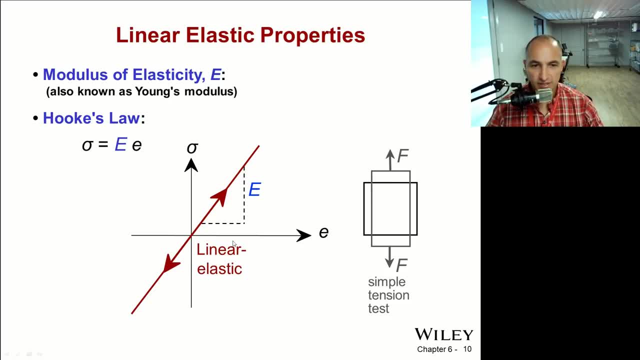 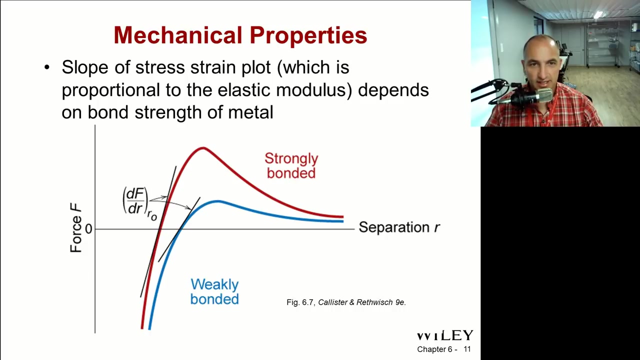 the slope of the stress versus strain to calculate the elastic modulus. so elastic modulus is just stress divided by the strain. from Hooke's law, stress is equal to Young's modulus times strain. so this is a sample in tension. so the elastic modulus is as I said. 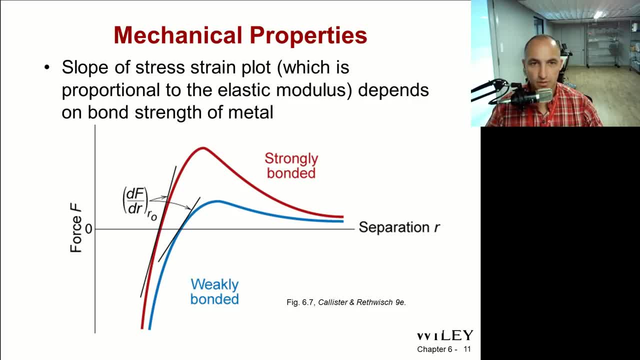 proportional to bond strain at all. so the slope- steeper slope- is going to be higher, elastic modulus, remember it's stress over the strain, so a higher change in stress over a smaller change in strain. so the red line here and the blue line is going to be: 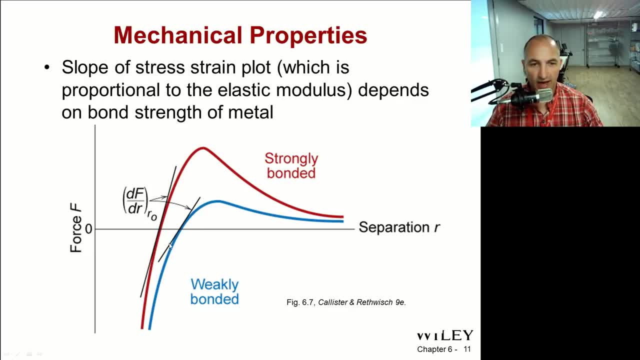 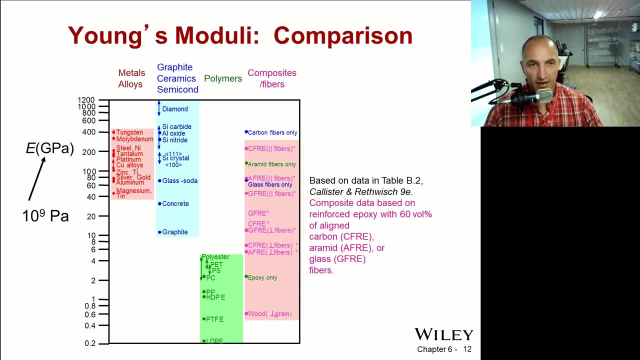 more weakly bonded where you have less of stress for strain or separation. so, looking at a variety of materials here for Young's modulus students are gigapascals in this graph, metals are tend to be very high and the ones here at the top, like tungsten and moly. 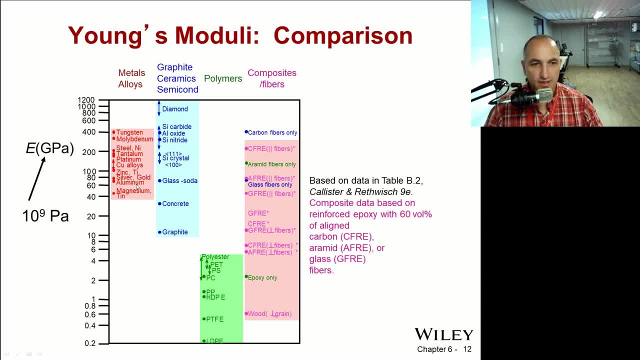 have a very high melting temperature, and magnesium and tin have a very low melting temperature, and so for metals, the Young's modulus is proportional to the melting temperature of the metal. so remember that the material melts when the bonds vibrate so much that they start to break. 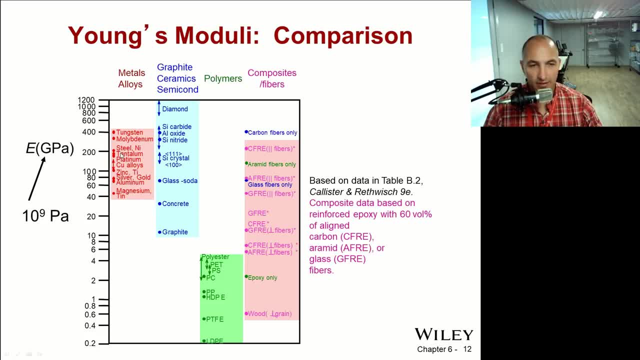 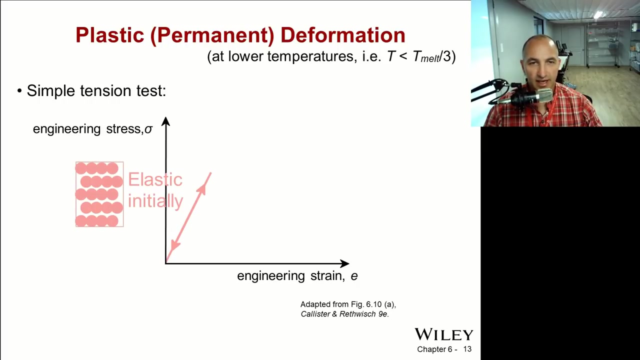 so that's the strength of the bonds, which is the Young's modulus. so diamond here wins the Young's modulus race. and our polymers don't do a very good job of that. they have very low Young's modulus. alright. so plastic is, as I mentioned previously. 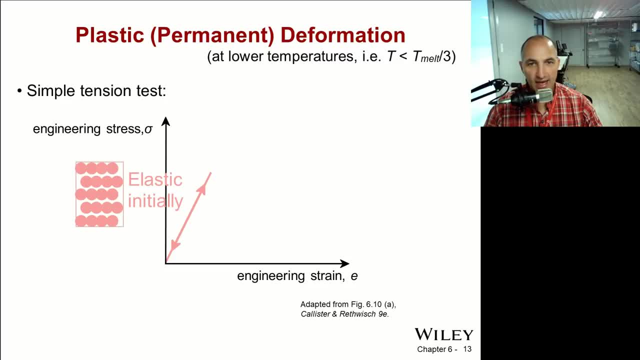 permanent plastic is permanent deformation and if we sample at a temperature less than a third of the melting temperature, this is lower temperatures. and put it in a simple tension: see, there's no shear here and we're stretching those atomic bonds and we can stretch and release the. 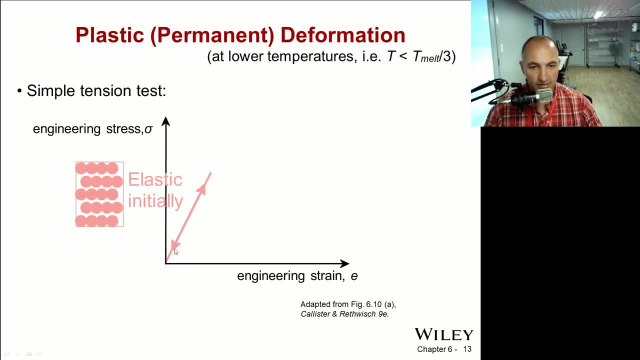 force on that indefinitely and it's just going to keep bouncing back and forth and return back to the origin here and we're going to see no permanent deformation. but if we start pulling the specimen harder then we're going to reach a point where atom planes start to slip. 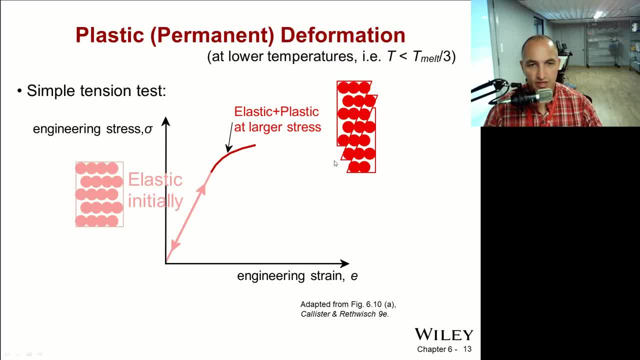 so this is going to be occurring at larger, like the earlier plot where it was force, now we're looking at strain. so but then if we release the specimen, leave all forces from it, we're still going to have some permanent or plastic deformation after the load is removed. 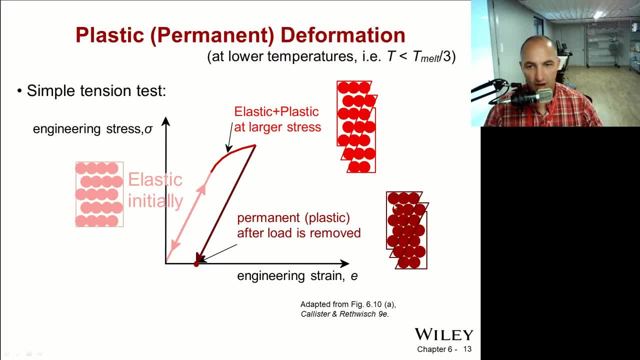 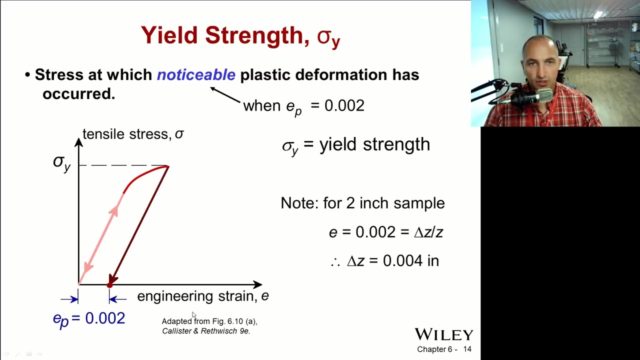 notice here that the atoms are not stretched anymore, so they bounce back, but you still are left with bones. that's the non-recoverable part. so the plastic strain on the sample is epsilon p or plastic strain now yield strength, another term here- and this is the. 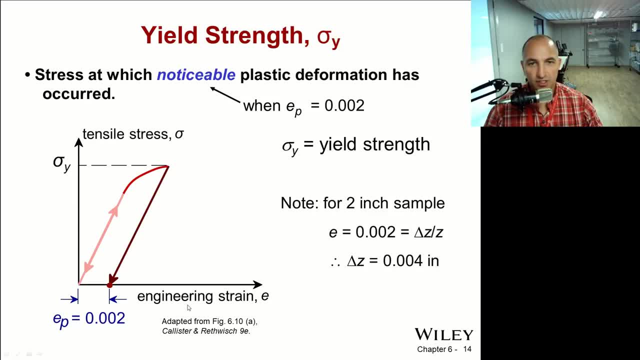 stress at which noticeable plastic deformation has occurred. so this is a material property. we can look up tables, just like young's modulus tables, for different materials with different yield strengths, and often we use a convention here with where we where the yield stress is measured at a 0.002. 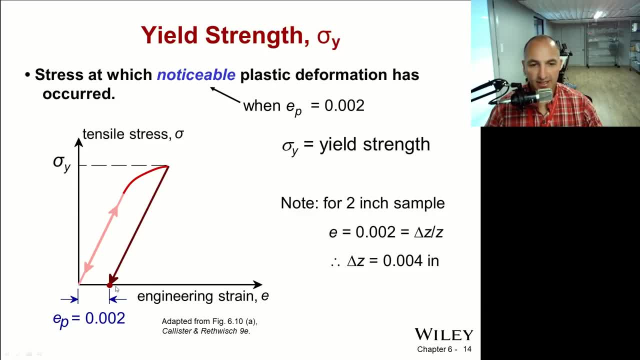 percent offset or engineering strain of 0.02, and that's normally that's needed because often it's very difficult to identify where the yielding has started because it's such a gradual transition between linear, elastic and plastic section. so if we were to have a 2 inch sample then 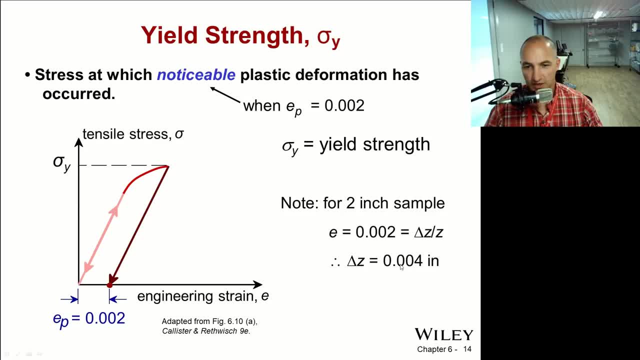 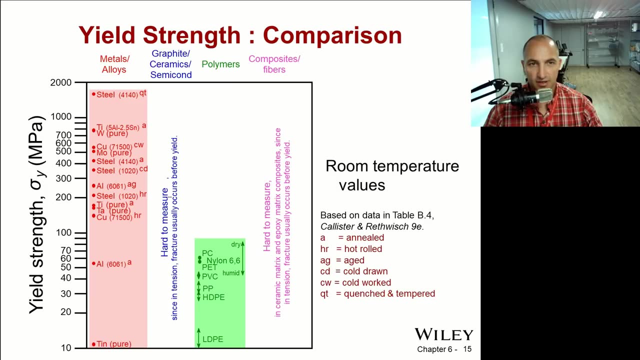 that's like measuring the yield when the sample has been stretched by 0.05 for 4 inches. okay, so that's the stress at which noticeable plastic deformation has occurred. so, just like young's modulus, we can look at value for yield. strength and steels are all over. 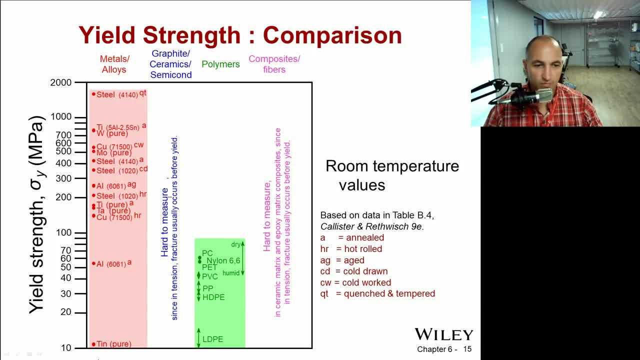 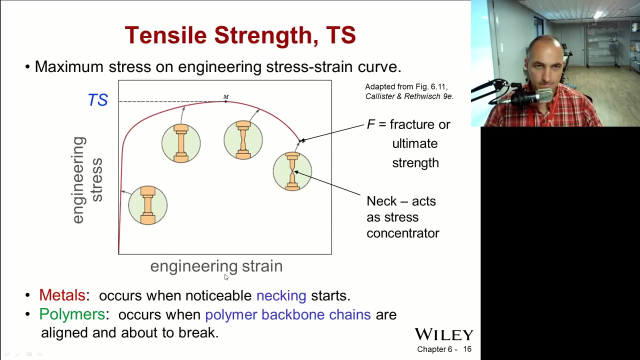 the map with yield strength. some of them like tin and some are very high like steel. 4140 quenched- chromoly quenched. it's even higher than very strong, very high yield for that one um. so polymers, another term is tensile strength, so tensile strength. 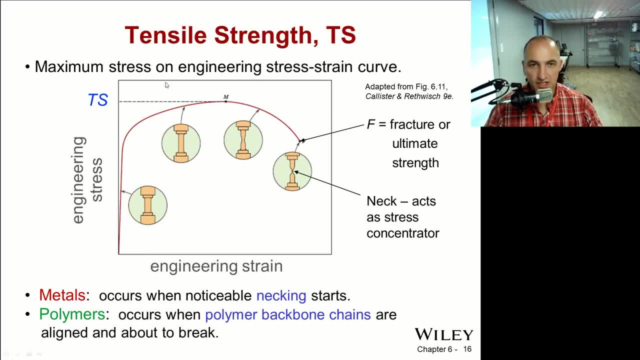 is the maximum stress on the engineering stress strain curve um, before it starts to drop back down again. now you may wonder: why does it drop back down? and the reason why is because the specimen starts to connect and, as you remember, stress is always calculated over original cross-sectional area. 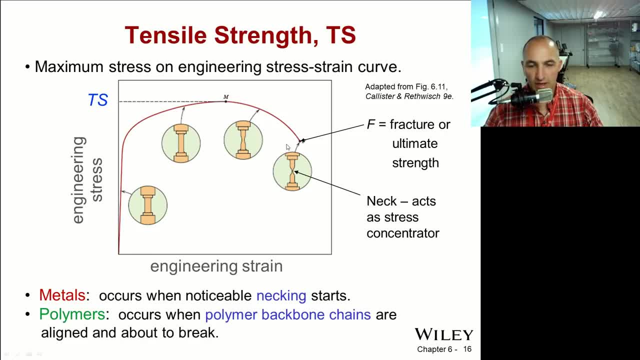 so in reality, what the sample is feeling at neck reach is a much higher stress than what is plotted here. but since this engineering stress strain curve and we're able to pinpoint maximum stress for this. so if we continue stretching it, we're going to get to the point where 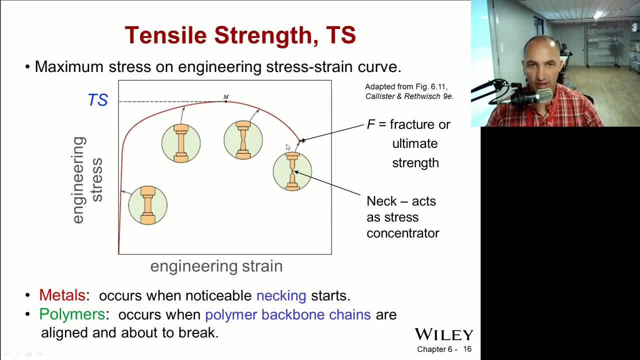 there's fracture and that's called the ultimate strength, another term from tensile strength. ultimate strength, or at which point at which the neck gets so thin and then the sample breaks. so for polymers, maximum tensile strength occurs when the polymer backbone changes are fully aligned. 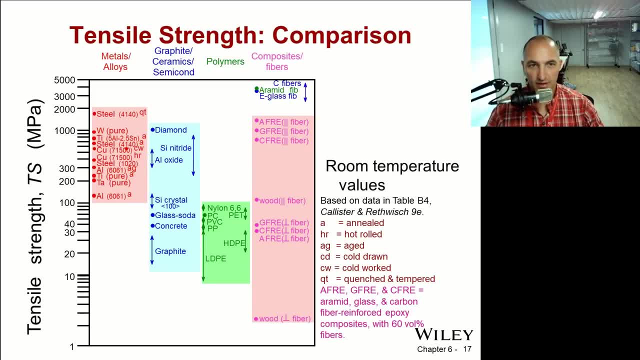 they're about to break. so, as you know, this is again a third material property: um, elastic modulus yield strength and now tensile strength. looking at different materials: metals and steel- very strong, 4140 tempered. and fiber- carbon fibers are very, very strong tension and they're way up there. 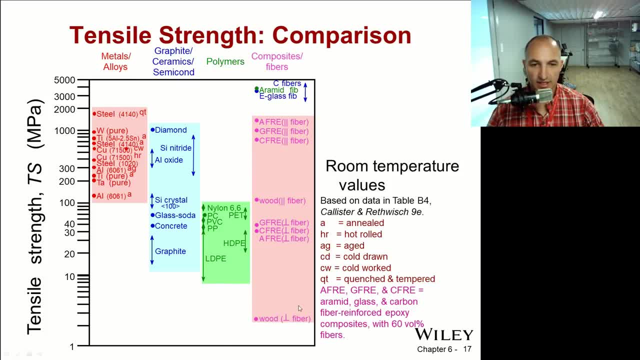 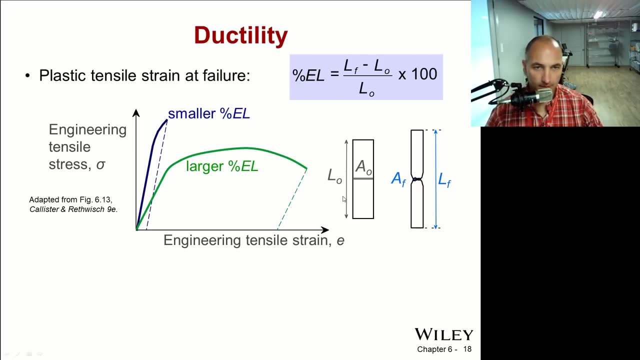 and wood is the worst for for tensile stress. another term that we know about materials and a material property is ductility. now ductility is measure of the elastic tensile strain failure, so it's called percent elongation. so that's the final length minus the original length. 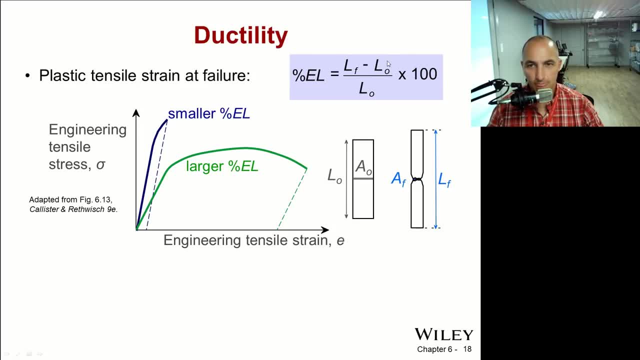 over change in length at the point of fracture over the. multiply that by one. so we have a sample here with a small ductility elongation and one that has a large ductility or elongation. so just because it might have a very high yield, strength, tensile strain. 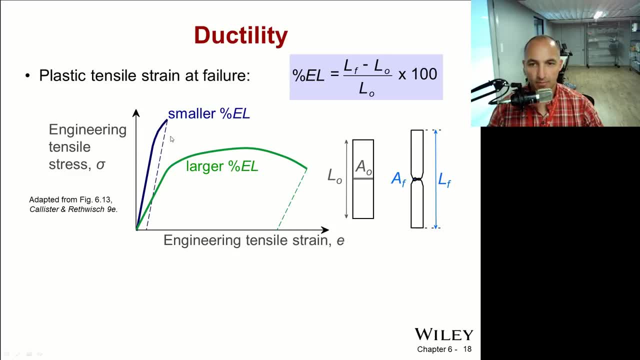 ductility. there's another ductility measurement that's synonymous to elongation and that's RA, which is reduction area. so that's original area minus the final cross-sectional area over the original cross-sectional area. so in a ductile sample we'll have necking, or necking that occurs. 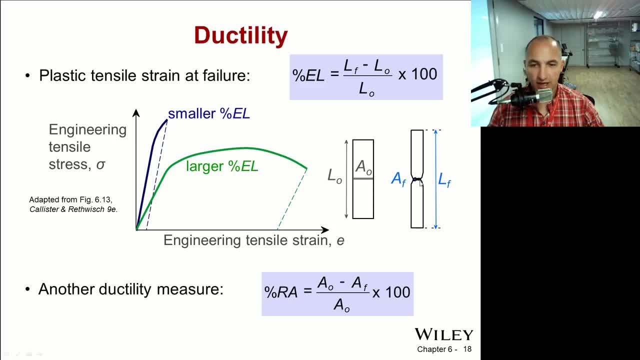 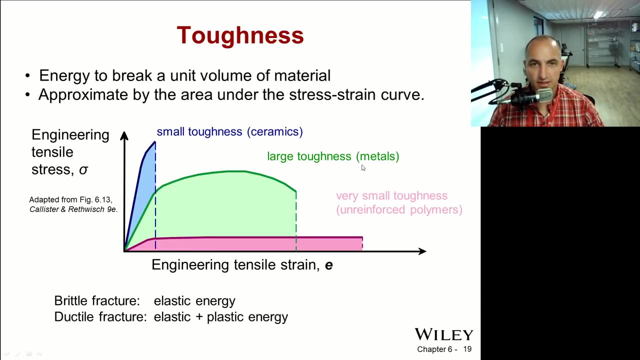 smaller cross-sectional area at the point of fracture and that will then have high ductility value associated with it. now, toughness is a great material property because it takes into consideration both the ultimate strength- tensile strength- and also the ductility. so an ideal sample will have: 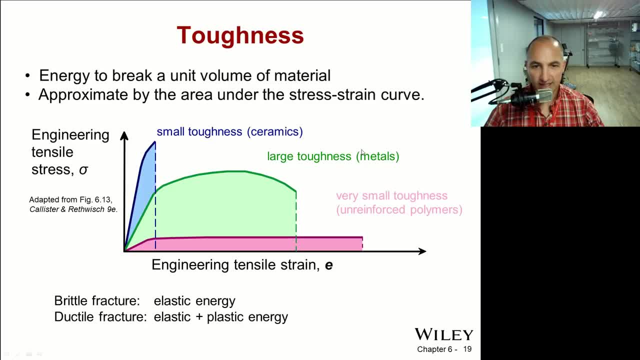 both high tensile strain and high ductility. that is going to be something very tough. that's what we mean by toughness. so it's the energy and volume of material and it's approximated by the area under the stress strain curve. so the green graph has the largest. 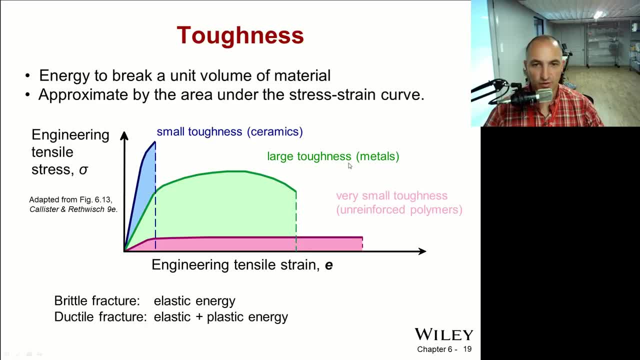 of cross-sectional areas, and so that is going to have the largest toughness. typically metals win out on these toughness measurements. brittle brittle materials tend to have various small toughnesses and polymers tend to have very small toughness. they might have great ductility, but the area under that 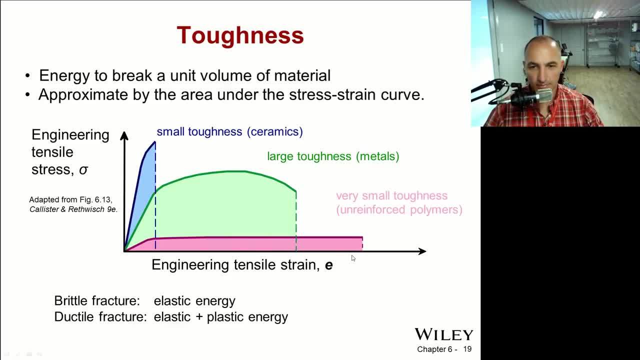 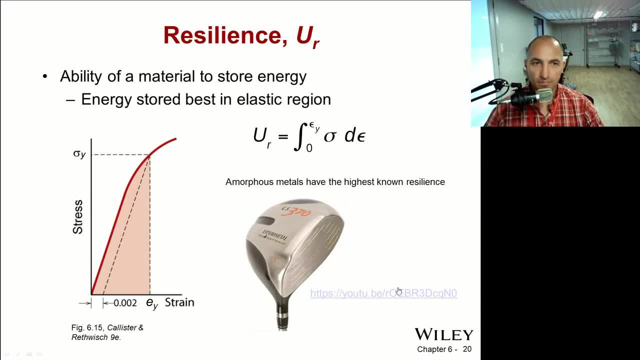 stress strain curve is going to be very small, so you'll have low toughness. now another material property that is important- not as important, but we call this resilience- and it's the ability for a material to store energy. and the ability to store energy is just the area under. 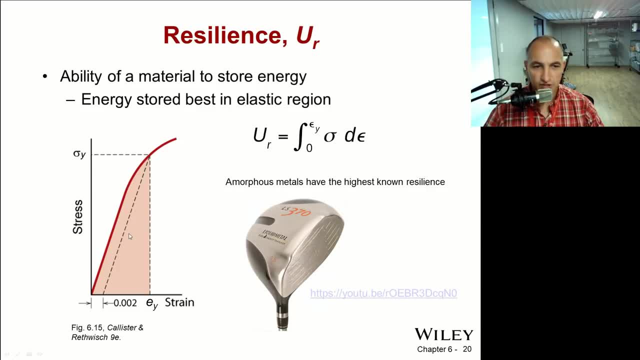 this linear elastic stress strain curve, and my father worked for a company called Liquid Metal and it used a very unique metal and it was an amorphous metal and it had the highest known resilience and I think they also made like baseball bats out of this amorphous metal as well. 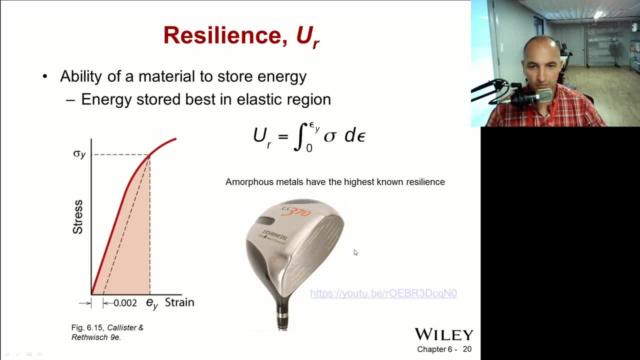 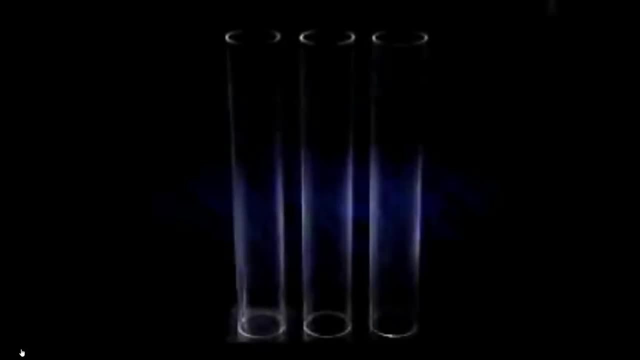 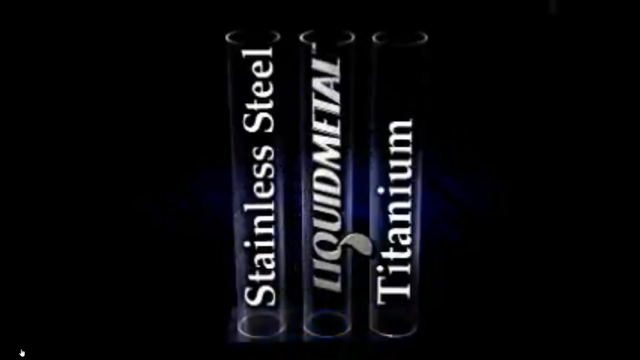 but I'd like to show you a short video of the on YouTube of how awesome this, this amorphous metal, is with their resilience. three tubes, three striking plates, a stainless steel surface, titanium and our own liquid metal alloy. three identical steel balls are dropped on the individual plates. 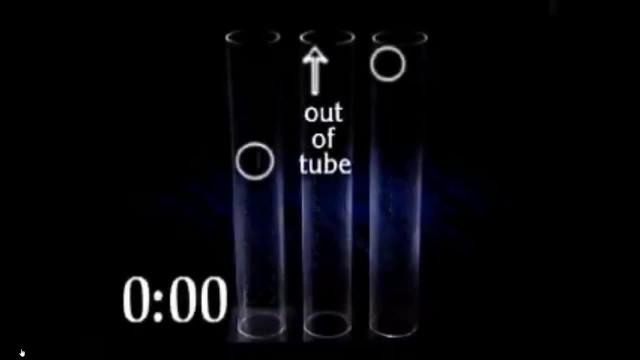 simultaneously liquid metal. a metallic glass has a very high elastic strain limit and, accompanying, very high strength. to put it simply, the high strain limit makes liquid metal the world's premier spring material. it's the best material we could possibly come up with to store and retrieve elastic energy in a mechanical 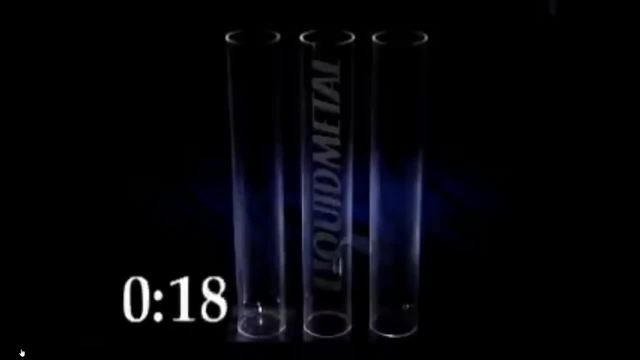 device, a material which can efficiently store energy and give it back again up to very high strain. a material which can store a very high density of elastic energy becomes the premier material when that performance benchmark is critical: any material which can efficiently store elastic energy up to very high densities. 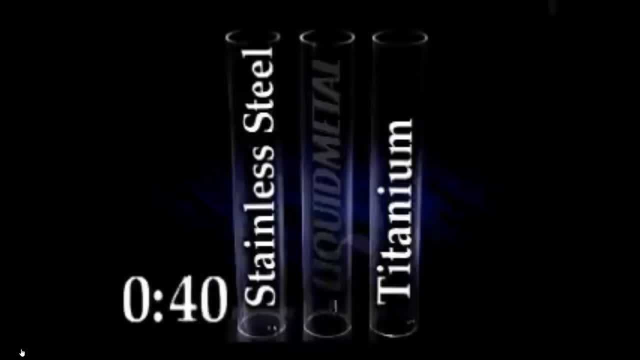 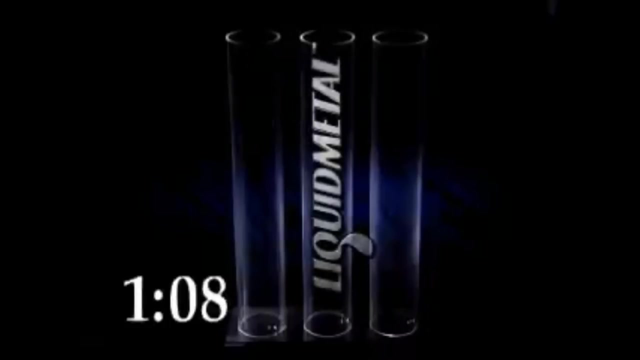 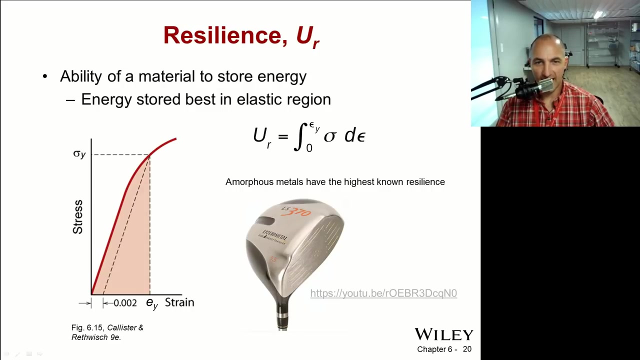 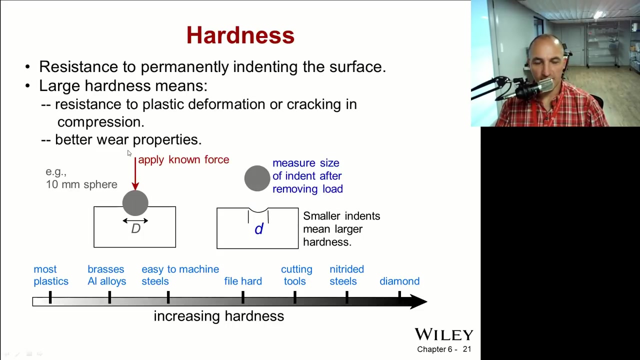 is superior to other materials in that respect, will be the premier material for those kinds of applications, the KAAS. so that's an example of a material with very high resilience. Another material property is called hardness, and this is resistance to plastically indenting the surface of the material. 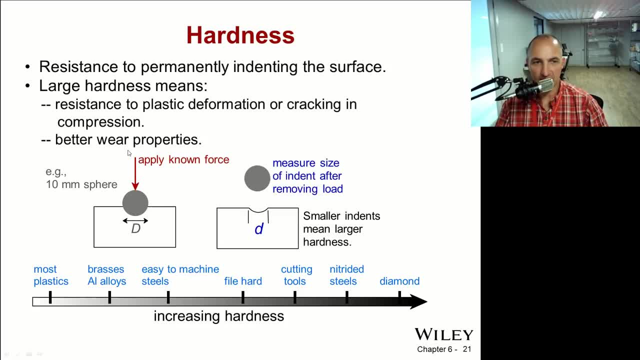 Large hardnesses mean the resistance to plastic deformation or cracking, while in compression and better wear properties. We have equipment in the materials lab which allows us to measure hardness. There's different types of hardness testers, depending on the types of surface, how hard they are, how soft they are. 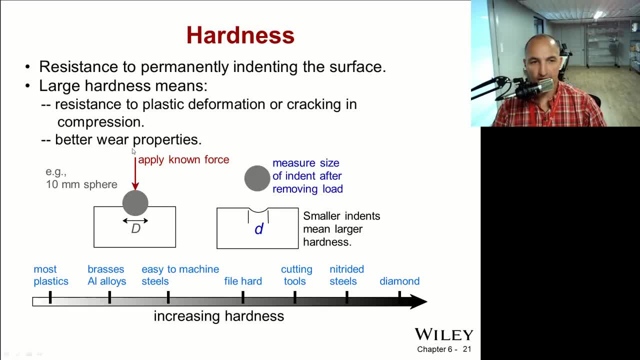 So we apply a known force and we measure the size of the indent after it's removed. So going from soft materials to very hard materials, Hard surfaces, plastics, then brass alloys and then easy machine steels like 1020 steel. then we have file hard steels which are high in carbon concentration, cutting tools, nitride. 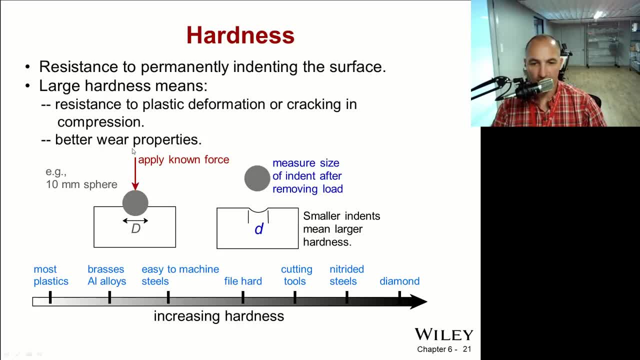 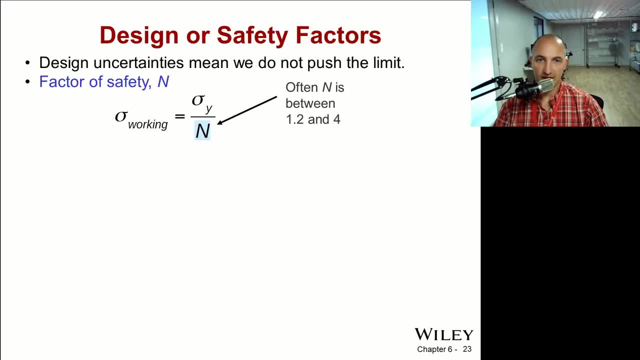 steels and finally diamond, one of the hardest known materials. Finally, we're going to mention here the design for safety factors. Okay, So there are design uncertainties, so there's also material uncertainties, So we don't want to push the limit, so what we do is we incorporate in a design factor. or a safety factor, and we call that. often it's between 1.2 all the way up to 4.. So there is an example here. Calculate a diameter D to ensure that yield does not occur in a 1045 carbon steel rod and. 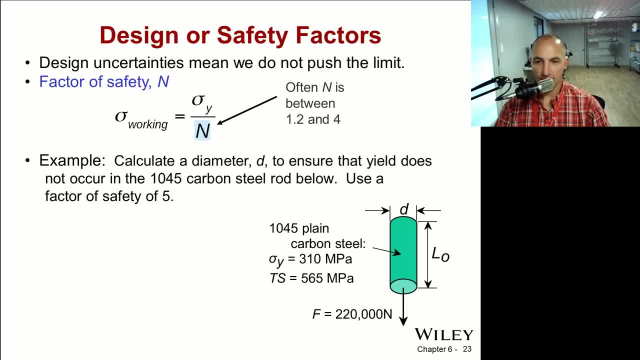 use a factor of safety of 5.. So here's our 1040 plain carbon steel from the table so we can look up, find that it has a yield strength of 310 megapascals and a tensile strength of 565 megapascals, and 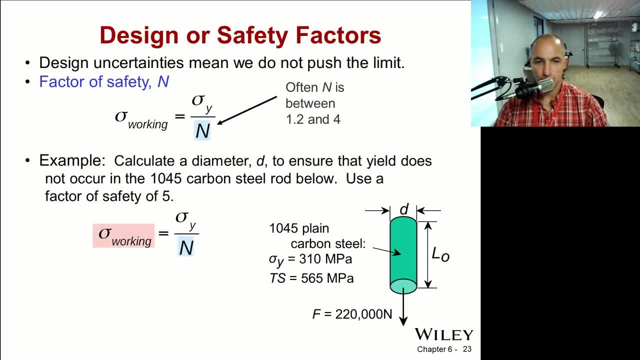 we are applying a force of 220,000 newtons, so we're plugging in a 5, and know that our diameter sample is 0.067 for 6.7 centimeters, And that is 0.067 for 6.7 centimeters. 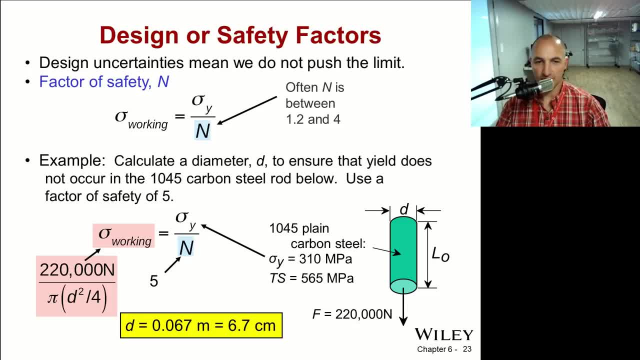 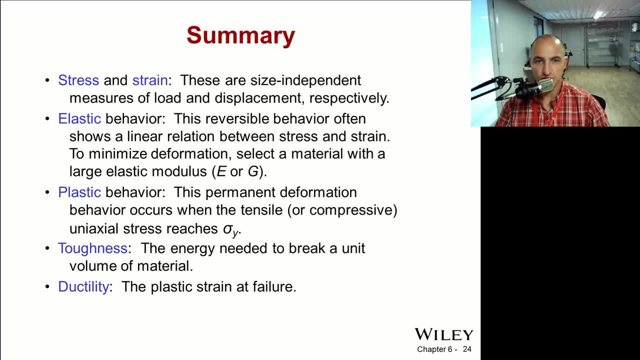 So, in summary, stress and strain, these are the size-independent measurements of load and displacement. So size-independent means that we divide it by the cross-sectional area or the length. Elastic behavior: This is the reversible behavior. Reversible behavior often shows a linear relation when stress and strain linear relation.